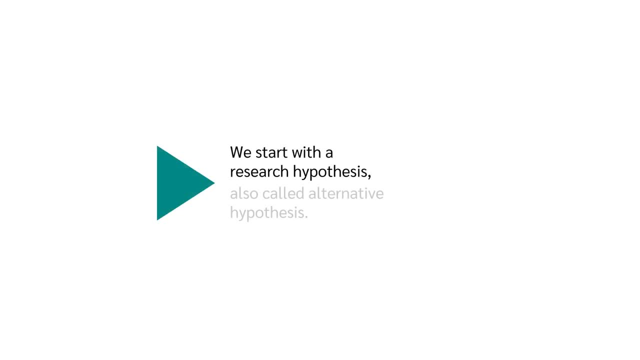 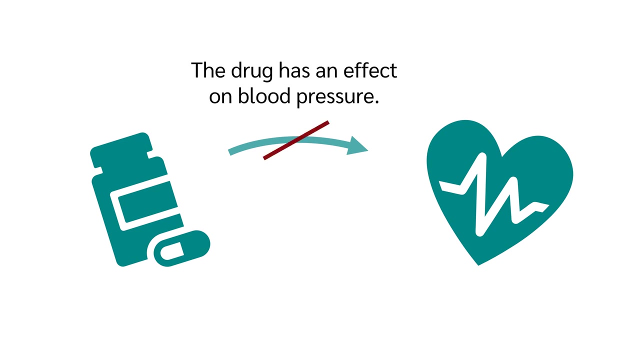 a hypothesis test, we start with a research hypothesis, also called alternative hypothesis. This is the hypothesis we are trying to find evidence for. In our case, the research hypothesis is the drug has an effect on blood pressure, But we cannot test this hypothesis directly. 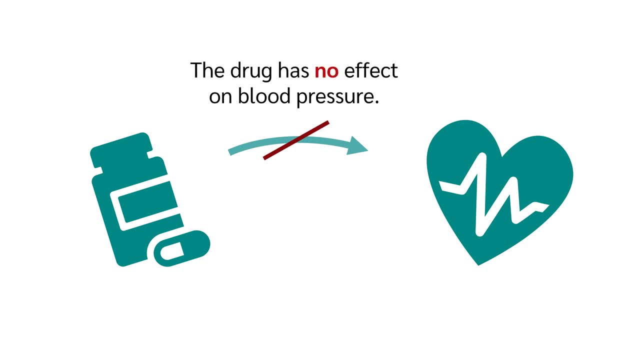 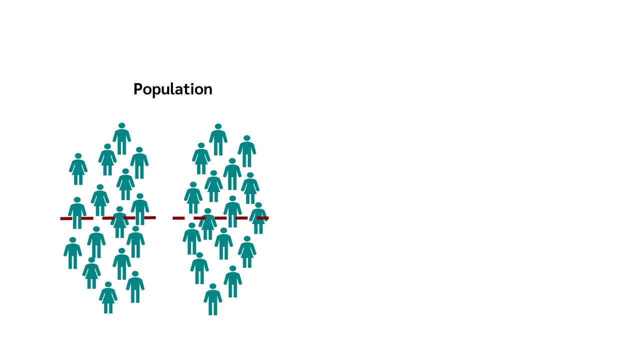 with a classical hypothesis test. So we test the opposite hypothesis, that the drug has no effect on blood pressure. But what does that mean? First, we assume that the drug has no effect in a population. We therefore assume that, in general, people who take the drug and people who do not take the drug have the 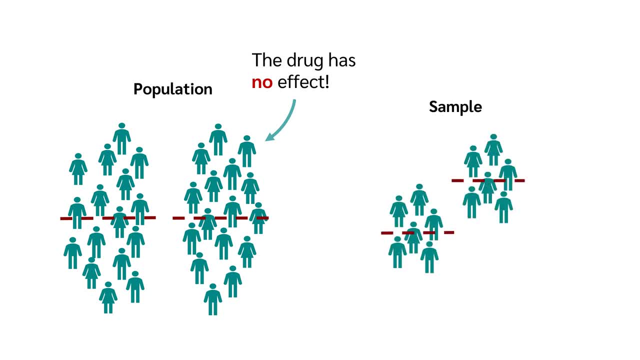 same blood pressure on average. If we now take a random sample and it turns out that the drug has a large effect in a sample- the再-l went a-leright back- then we can ask how likely it is to draw such a sample or one that deviates even more if the drug 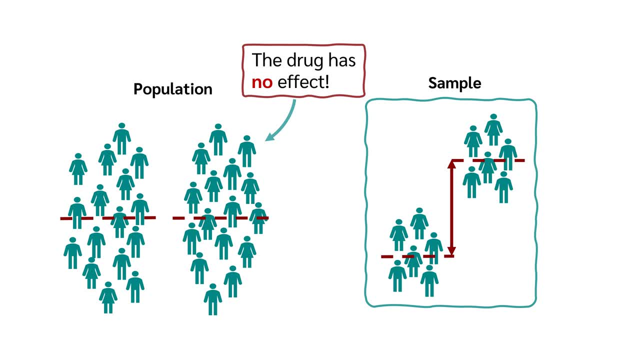 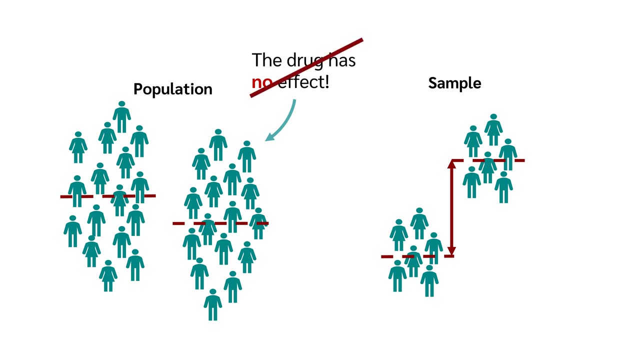 actually has no effect. So in reality, on average, there is no difference in the population. If this probability is very low, we can ask ourselves: maybe the drug has an effect in the population and we may have enough evidence to reject the null hypothesis that the drug has. 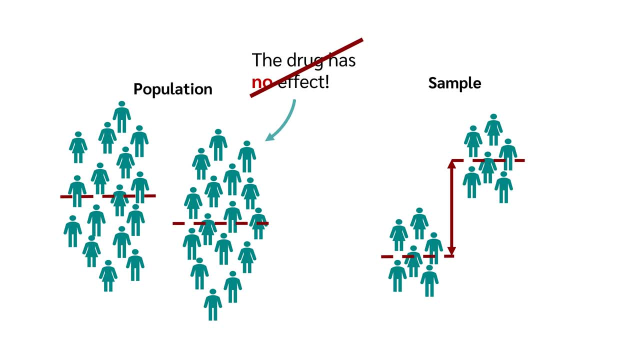 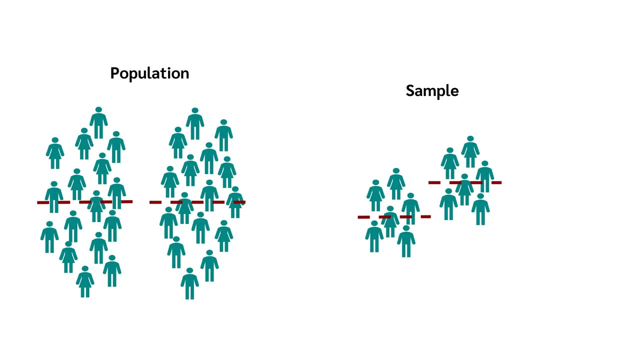 no effect, And it is this probability that is called the p-value. Let's summarize this in three simple steps. Number one: the null hypothesis states that there is no difference in the population. Number two: the hypothesis test calculates how much the sample deviates from. 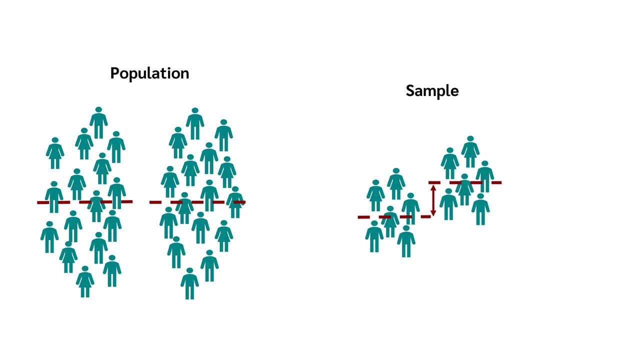 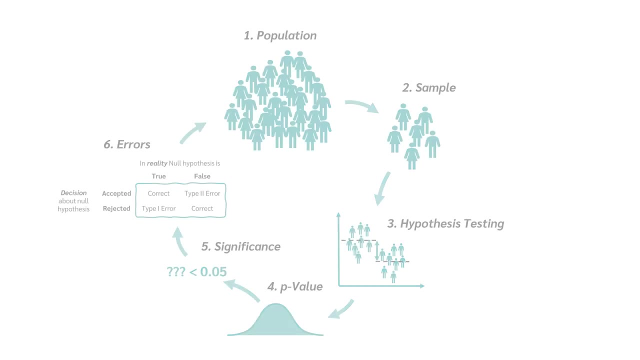 the null hypothesis. Number three: the p-value indicates the probability of getting a sample that deviates as much as our sample, or one that even deviates more than our sample, assuming the null hypothesis is true. But at what point is the p-value small enough for us to reject the null hypothesis? 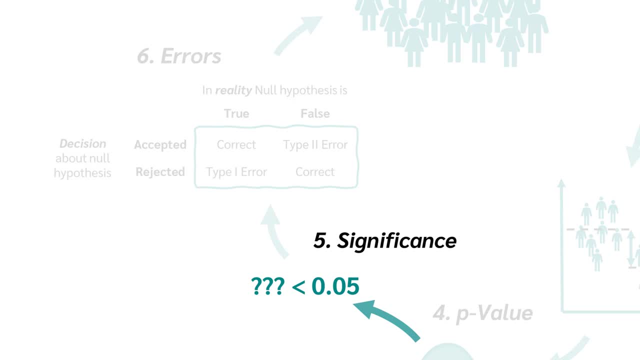 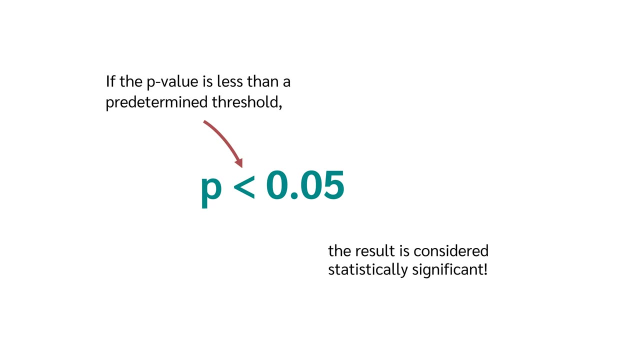 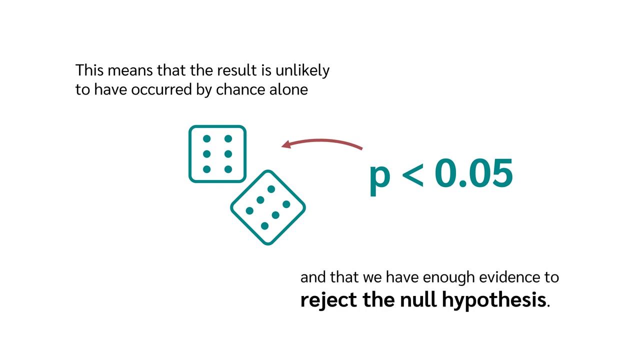 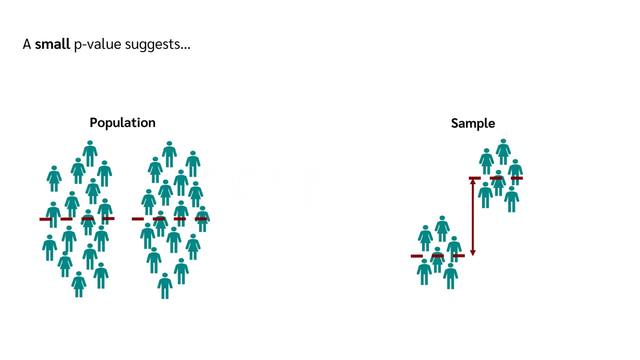 This brings us to the next point: statistical significance. If the p-value is less than a predetermined threshold, the result is considered statistically significant. This means that the result is unlikely to have occurred by chance alone and that we have enough evidence to reject the null hypothesis. This threshold is often 0.05.. Therefore, a small p-value suggests: 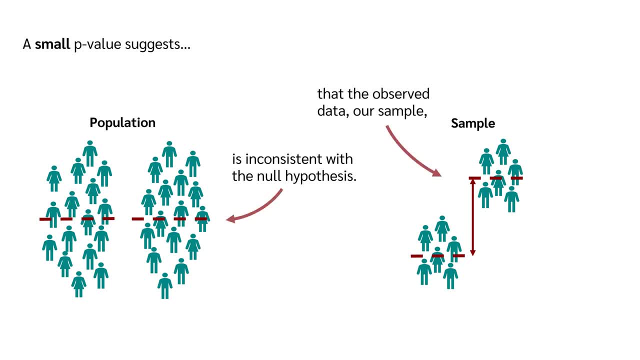 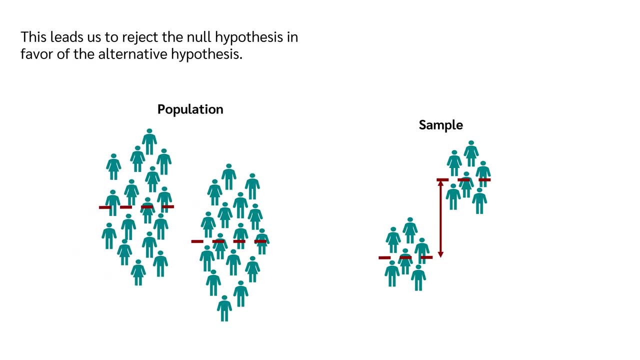 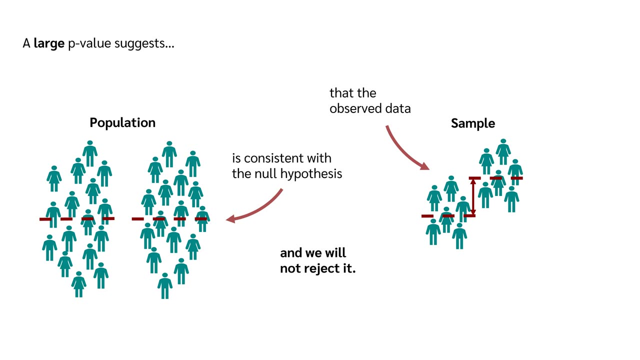 that the observed data- our sample- is inconsistent with the null hypothesis. This leads us to reject the null hypothesis in favor of the alternative hypothesis. A large p-value suggests that the observed data is inconsistent with the null hypothesis and we will not reject it, But note: 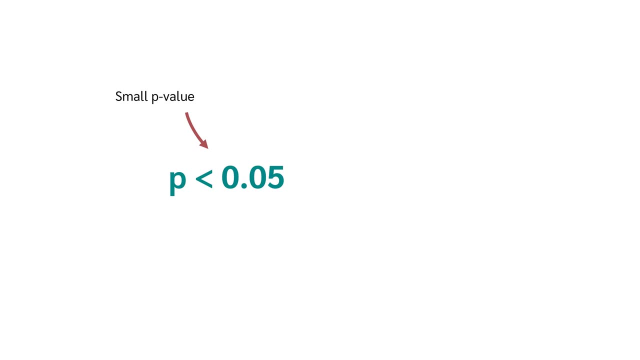 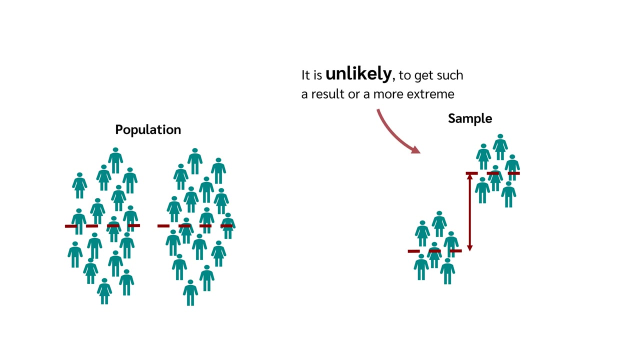 there is always a risk of making an error. A small p-value does not prove that the alternative hypothesis is true. It is only saying that it is unlikely to get such a result or a more extreme when the null hypothesis is true. And again, if the null hypothesis is true, there is no difference in the population. 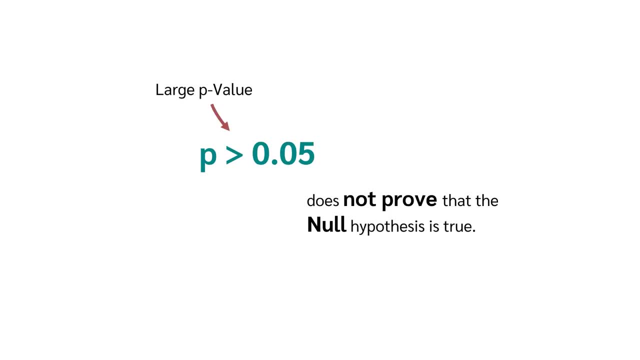 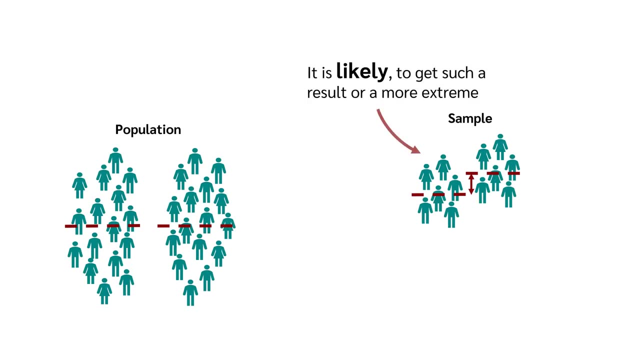 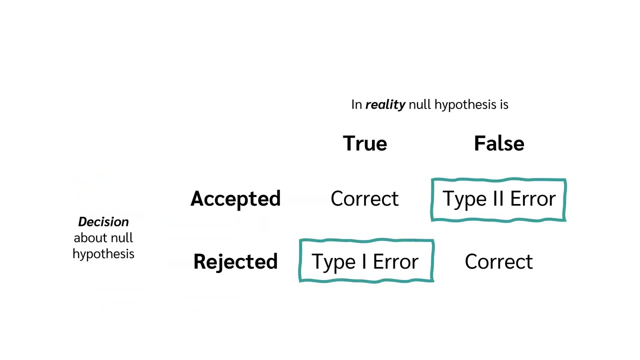 And the other way around. a large p-value does not prove that the null hypothesis is true. It is only saying that it is likely to get such a result or a more extreme when the null hypothesis is true. So there are two types of errors, which are called type 1 and type 2 error. Let's start. 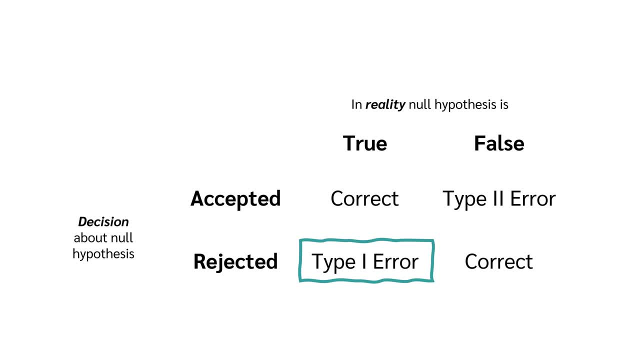 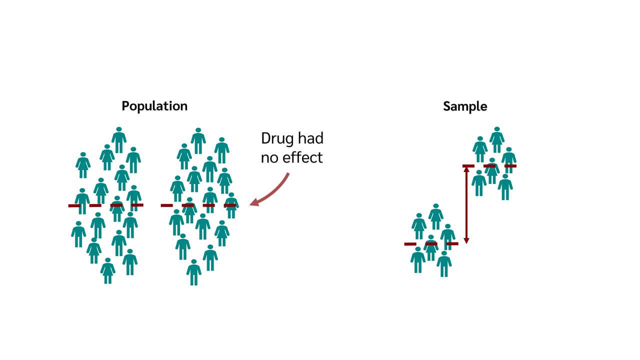 with the type 1 error In hypothesis testing. a type 1 error occurs when a true null hypothesis is rejected. So in reality the null hypothesis is true, but we make the decision to reject the null hypothesis. In our example, it means that the drug actually had no effect. so in 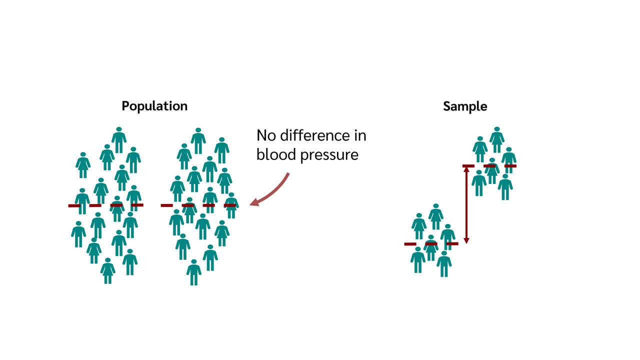 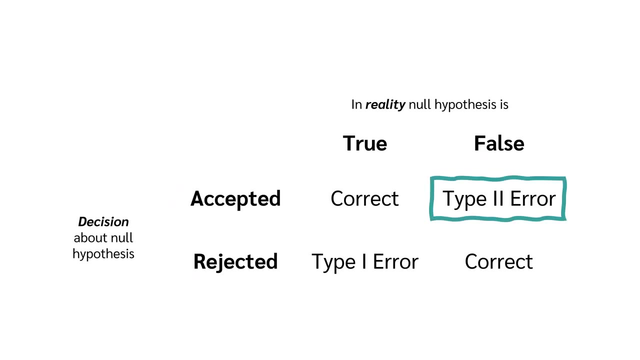 reality, there is no difference in blood pressure whether the drug is taken or not. the blood pressure remains the same in both cases. But our sample happened to be so far off the true value that we mistakenly thought the drug was working, And a type 2 error occurs when 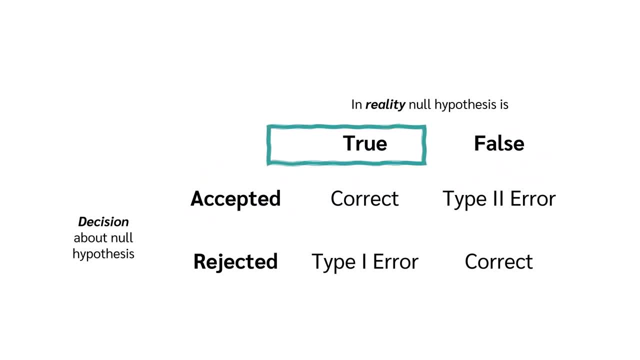 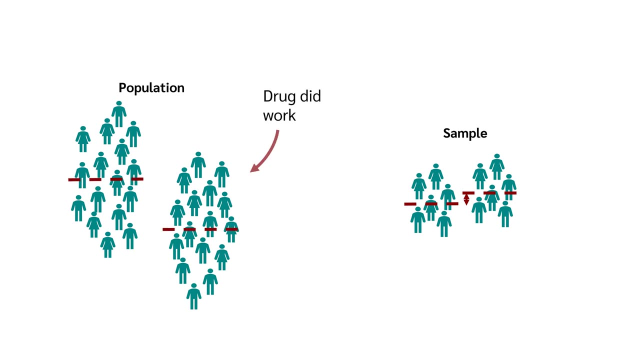 a false null hypothesis is not rejected. So in reality, the null hypothesis is false, but we make the decision not to reject the null hypothesis. In our example, this means the drug actually did work. there is a difference between those who have taken the drug and those who have not, but it was just a coincidence that the 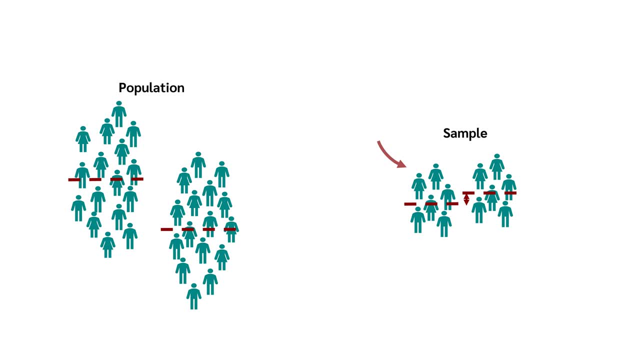 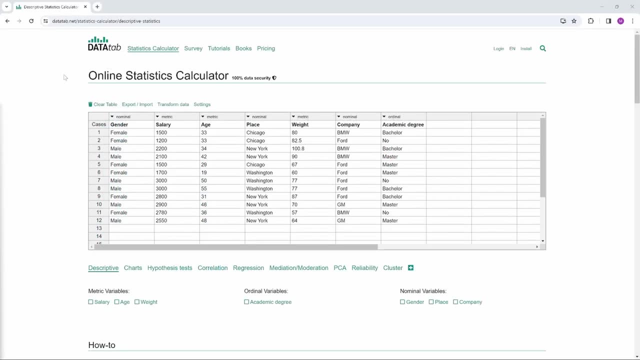 sample taken did not show much difference and we mistakenly thought the drug was not working. And now I'll show you how Datadep helps you to find a suitable hypothesis test and, of course, calculates it and interprets the results for you. Let's go to datadepnet and copy your own data in here. We will just use this example.